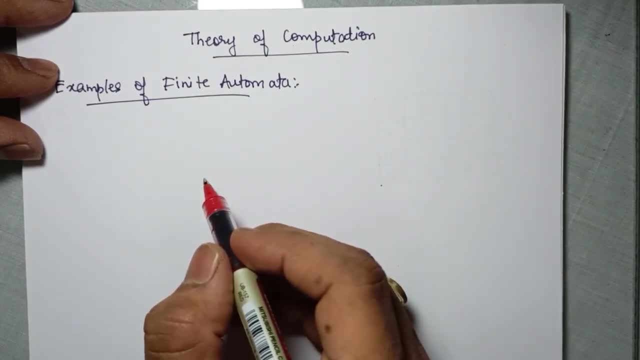 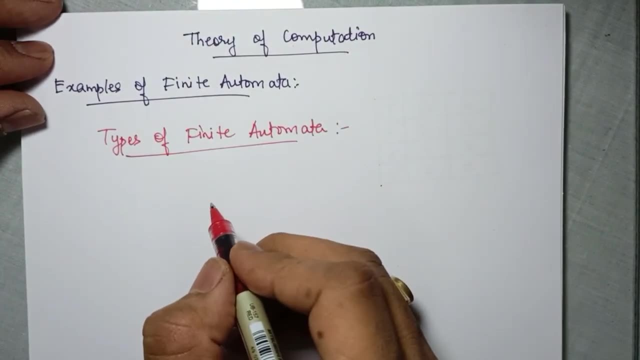 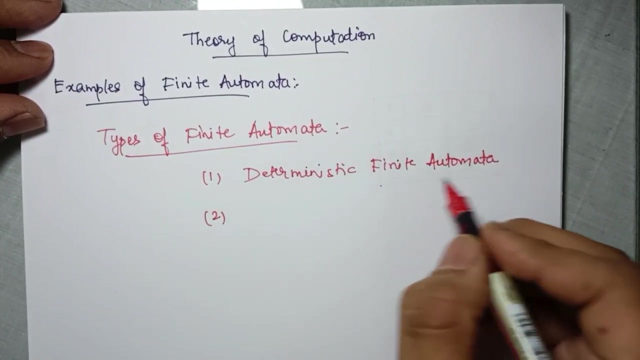 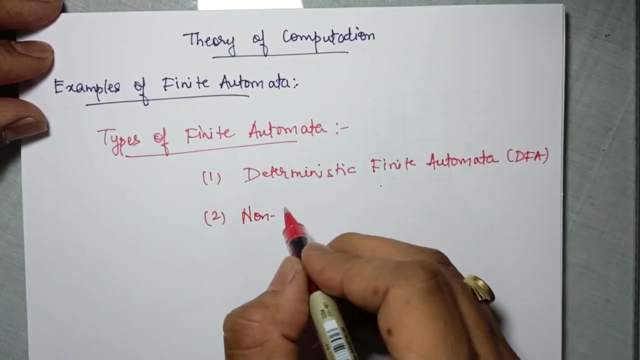 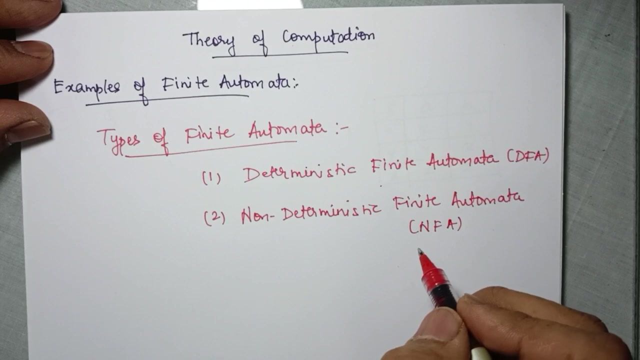 finite automata. let us try and understand how many types of finite automata are there. Basically, there are two types of finite automata: A deterministic finite automata, abbreviatedly called as DFA, and non-deterministic finite automata, abbreviatedly called as NFA. My dear friends, now, what is the difference between the deterministic 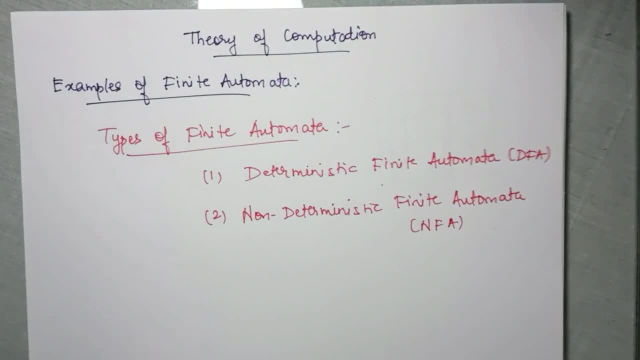 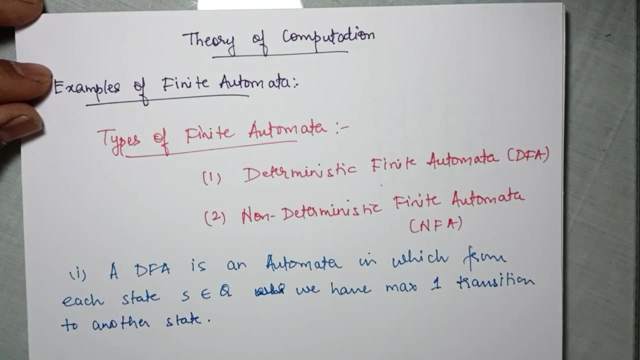 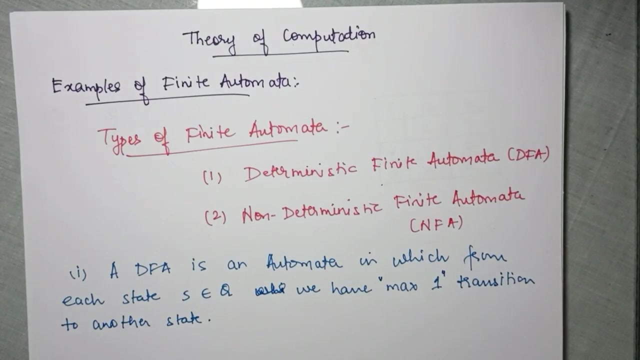 finite automata and the non-deterministic finite automata. So DFA is an automata in which from each state S that belongs to Q, we have maximum one transition to another state. That means from any given state. if you read an alphabet, 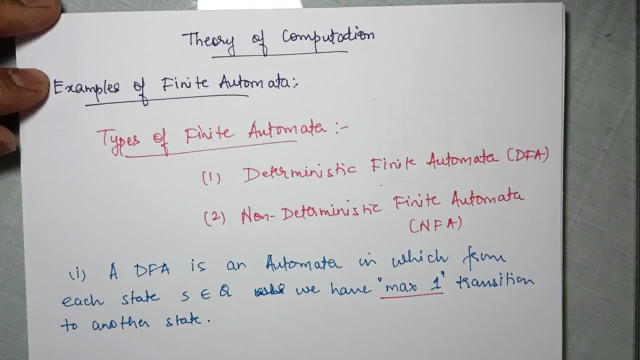 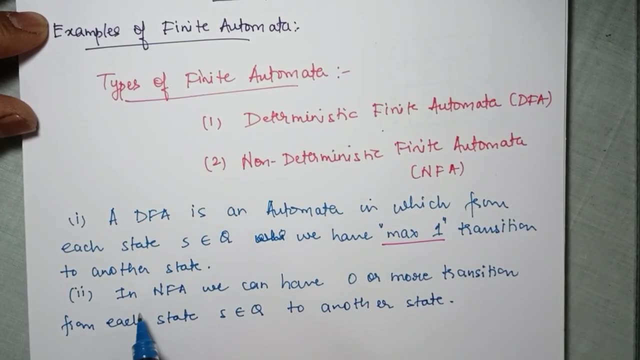 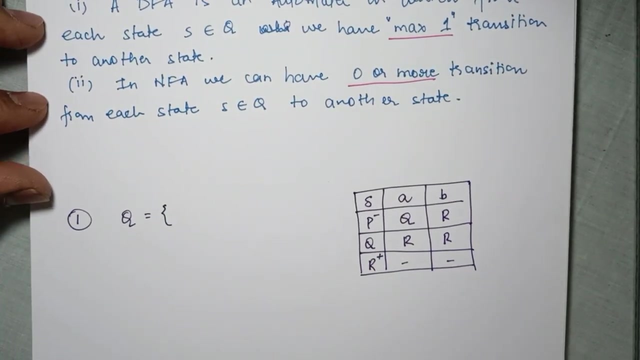 from the alphabet set you can reach maximum one another state, While in NFA we can have zero or more transitions. So DFA is an automata in which from each state S that belongs to Q to another state. This will get more clear when we will see example. 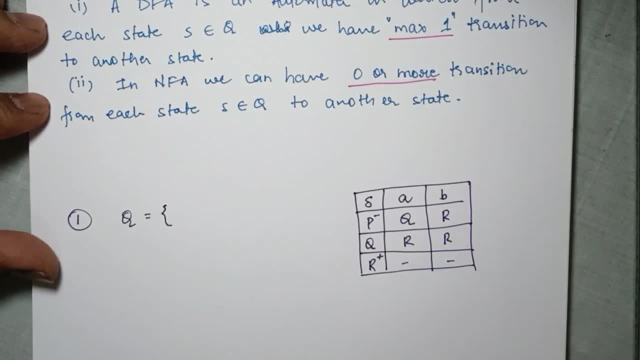 So, my dear friends, here is an example given for a finite automata. Let us see some details about this automata. This table given is called DFA. This table is called a transition table. My dear friends, the example given here is having this transition table. Let us understand. 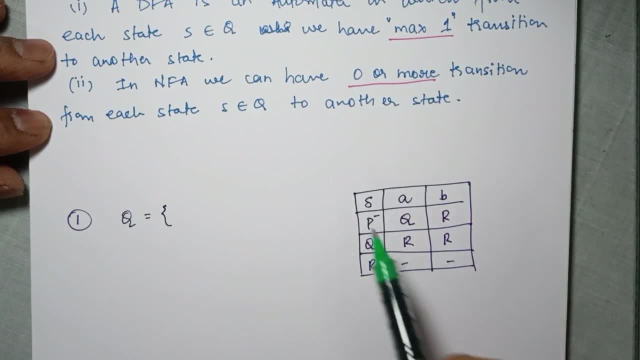 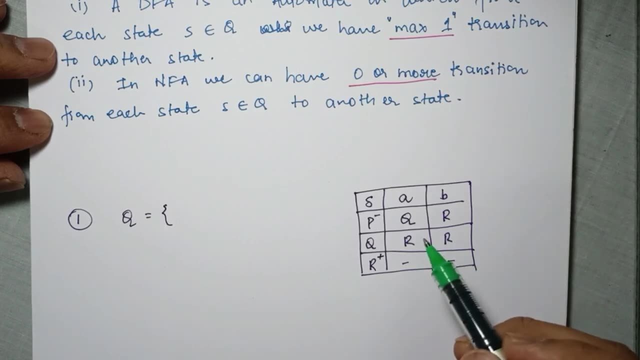 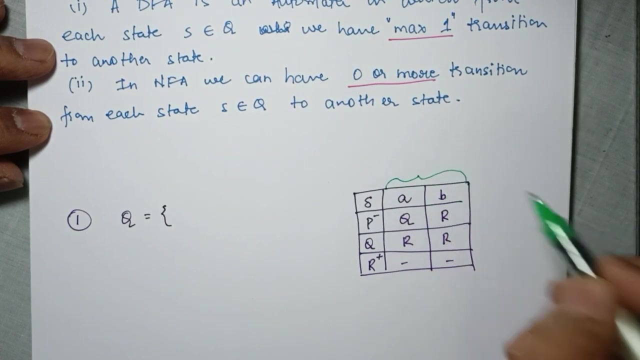 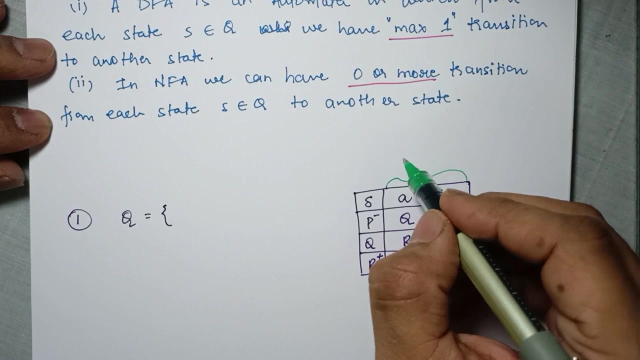 what this transition table means. And from this transition table, delta, let us try to have all the tuples that were given that we have for a finite automata Here. the tuples that are there in the row are the alphabets from the alphabet set, sigma And the letters. 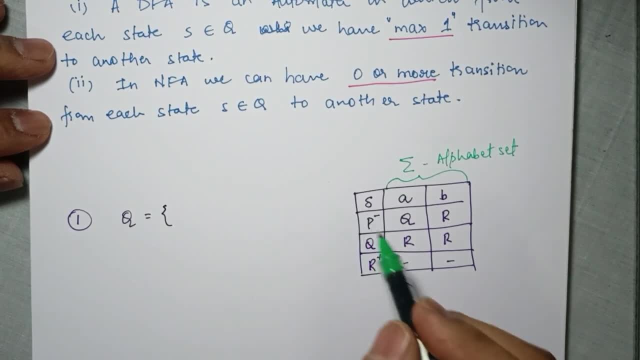 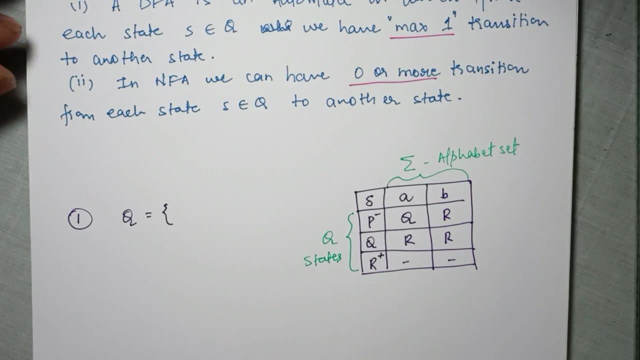 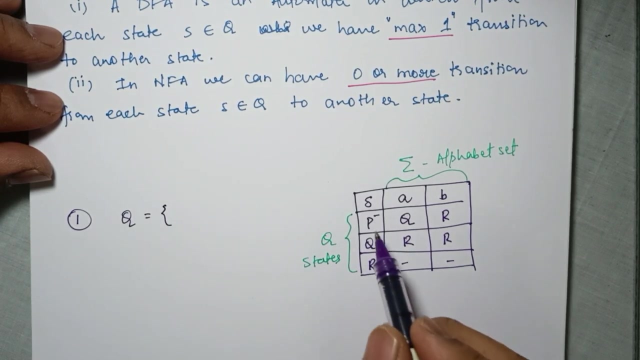 in the column here indicates the states that are there in the finite automata. So from this what I can see is that we have in the set Q. that is nothing but the set of states. we have P, Q & R. Then, if you remember the 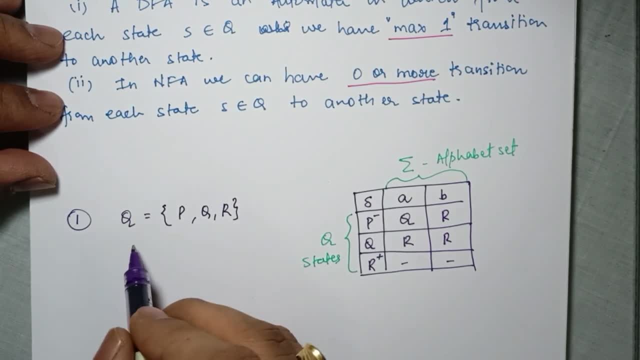 tuple of the finite automata. here we have in the alphabet set our singe. Now we have the alphabet set sigma containing two alphabets or symbols, namely A and B. Then we have the initial state QZ. Next we have the final state QZ, in which we have only one alphabets. 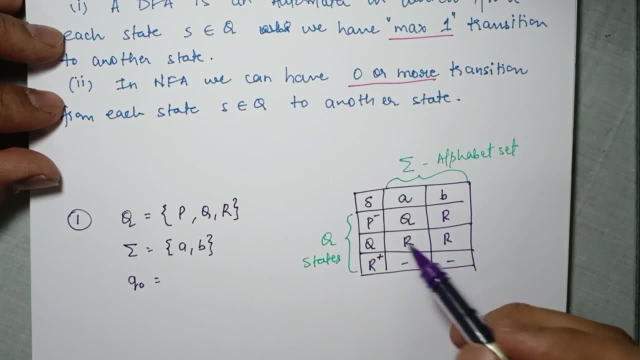 And after Mango, 독yr phlegm. QZ. psn. rules governing on one alphab: dönerيم. else we have the initial state QZ Void q0. now look at this table, my dear friends. here there are two states indicated with a. 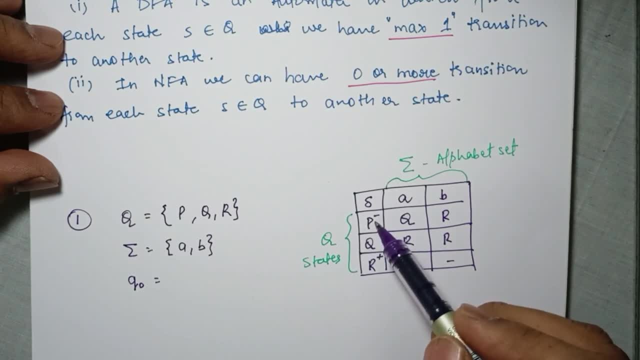 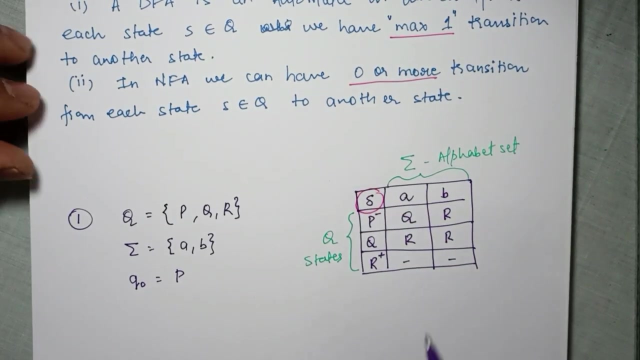 special symbol. so this minus sign indicates that it is the initial state. so my initial or the starting state for this given automata is p. then, my dear friends, we have the transition table, which is already given here. that is nothing but this delta, and last we have the set of final. 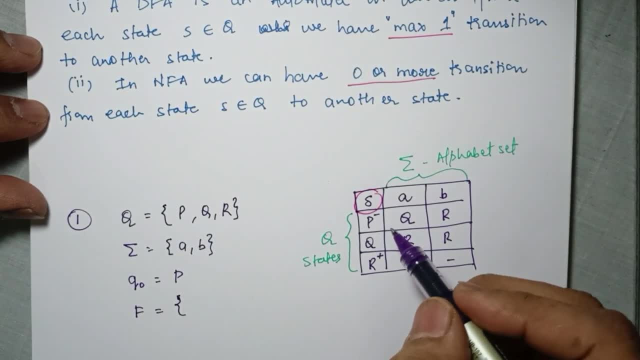 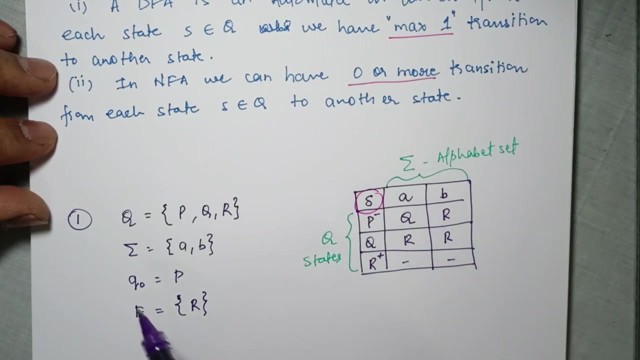 states f. so here, my dear friends, this state r, which is indicated by a plus symbol, is nothing but the final state. so in this finite automata, we have the set of states as p, q and r, the alpha set as A and B, the initial state as P. this is the transition table given and 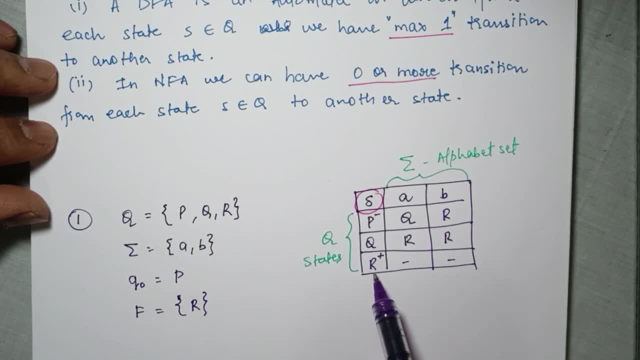 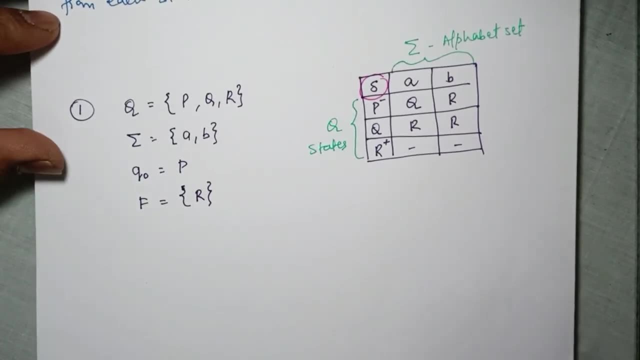 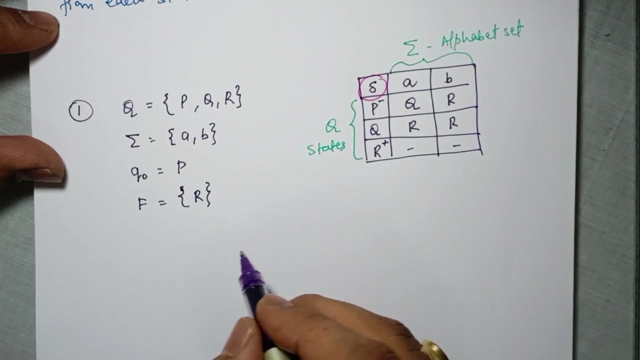 the final state is only R, but there can be more than one final state, as per the definition. now this finite automata can be drawn in a pictorial way where the states are represented as PQR: the initial state is represented by a minus sign, the final state is represented by a plus sign. then, from this transition, 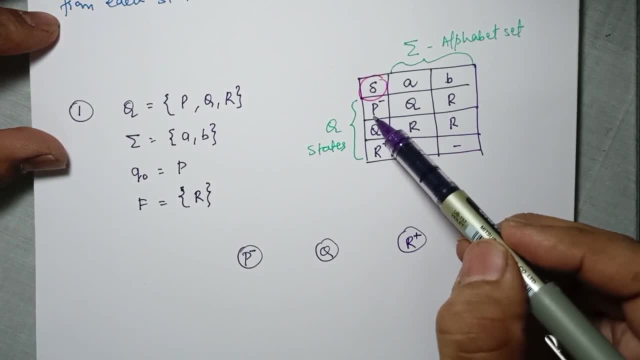 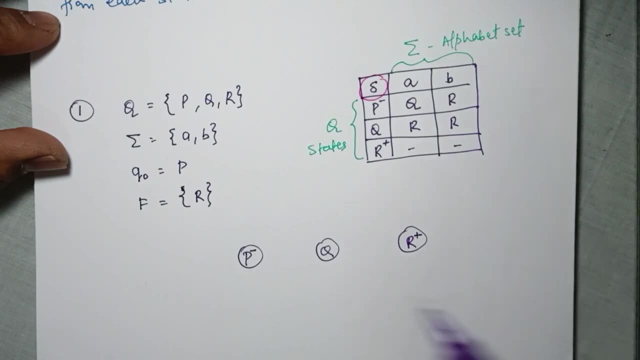 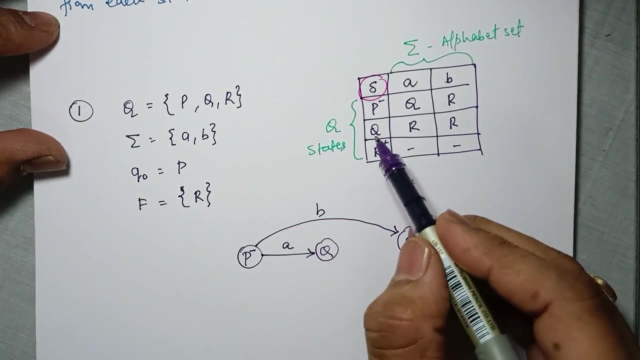 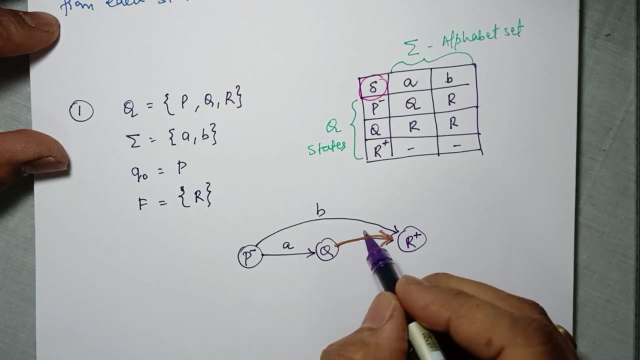 table. we can see that from the state P, if I read the alphabet A, I am going to the state P, Q. from state P, by reading the alphabet B, I am going to the state R. then from state Q, if I read A, I am going to the state R. from state Q, if I read B, I am going to the. 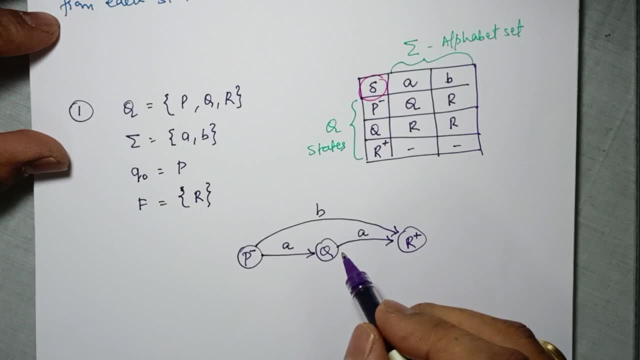 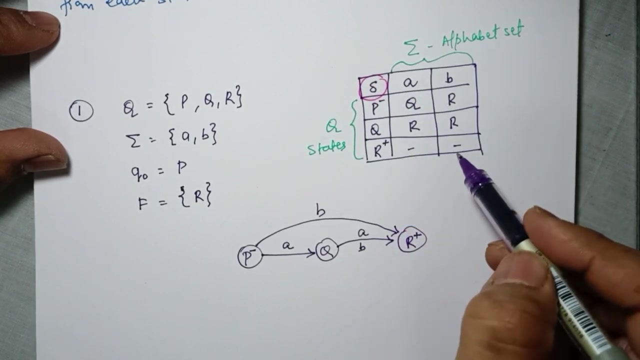 state R itself. so there are two ways of doing this. either I can draw another arrow or I can write here B on the same arrow. that makes no difference. now from the state R on reading A and B, there are no transitions. so that means this is my deterministic finite automata. 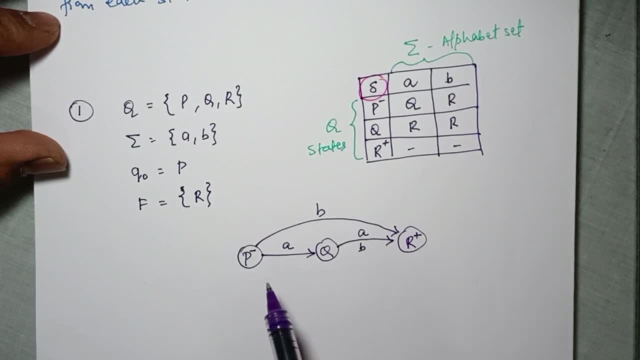 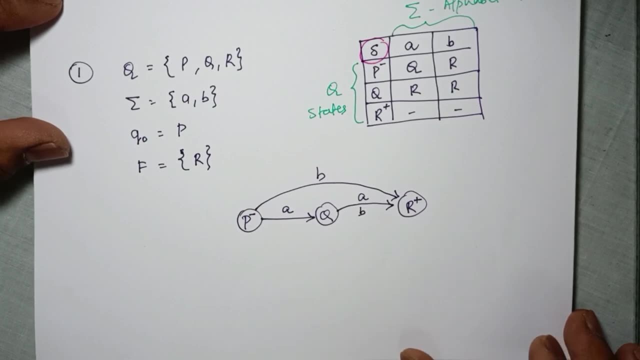 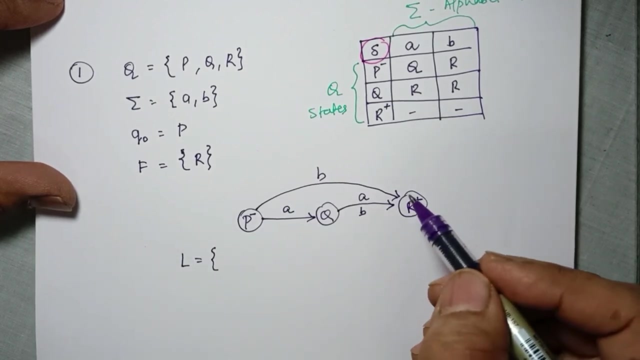 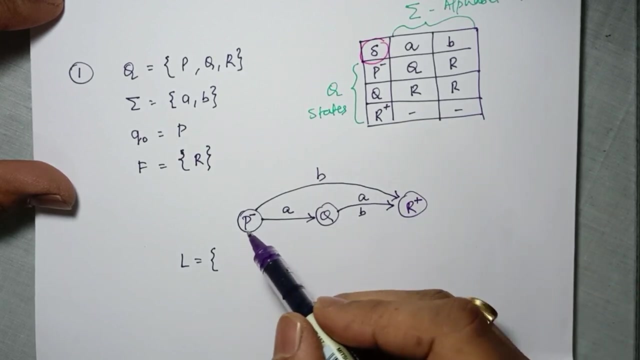 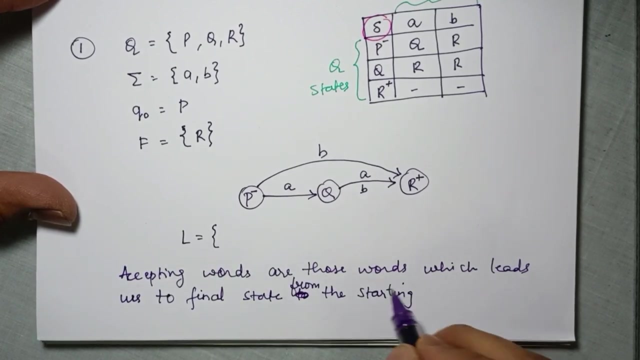 because from each state I am having maximum one transition to another state. now my term design. here we will play a completed version which is already defined. what I have done is for the changes generated by default. I can write a state T when I want to enter. I can draw aning and division, simply changing these. 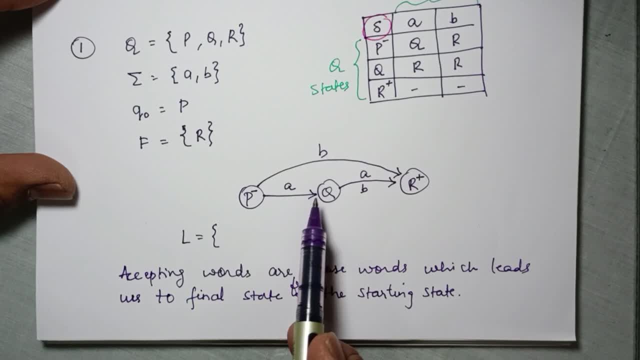 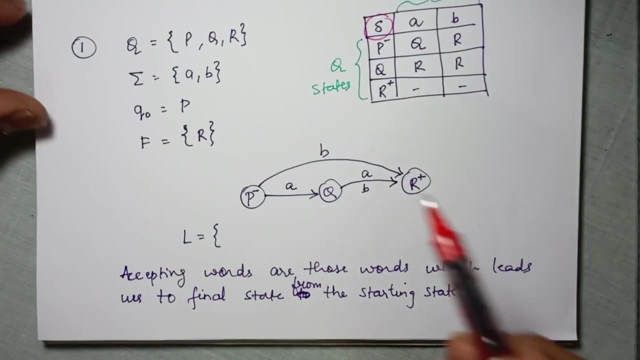 changes. so blink mắc turns our learning methods into thermodynamic conditions, and when you need some BOP or behavior, nothing but are those words which leads us to the final state from the starting state. So here let us see all the words that are possible. 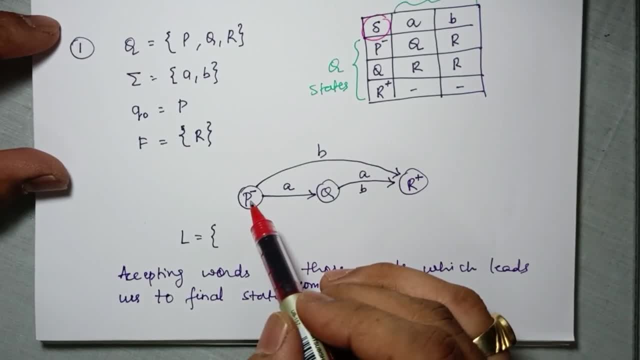 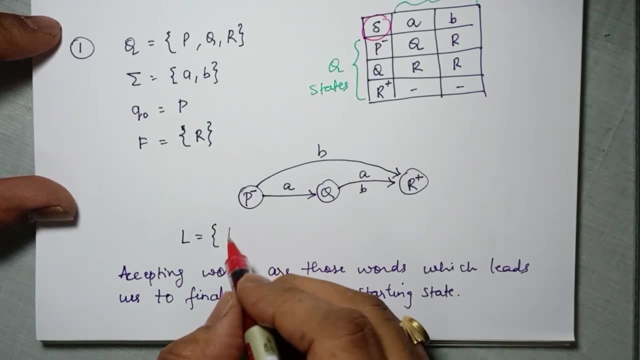 So if I see from here, P is my starting state. So if I read B, I am going to the state R, which is the final state. So the word B is accepted here From P. if I read A, I am going to the state Q, But Q is not a final state. 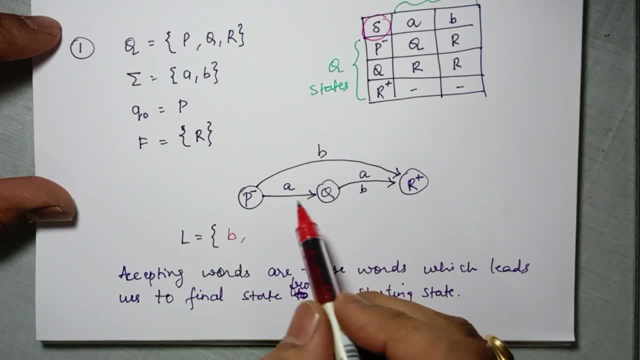 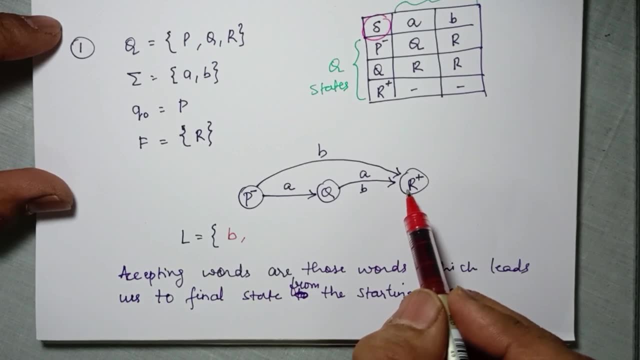 So my single letter A will not be accepted. But from state Q, if I read A, I am going to the state R, which is the final state. So, my dear friends, from starting state P, if I read A and A, I will go to the final. 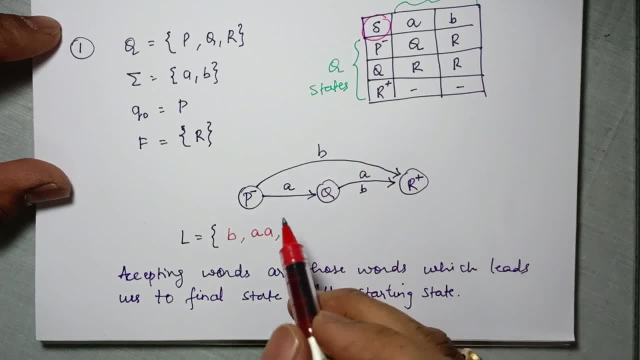 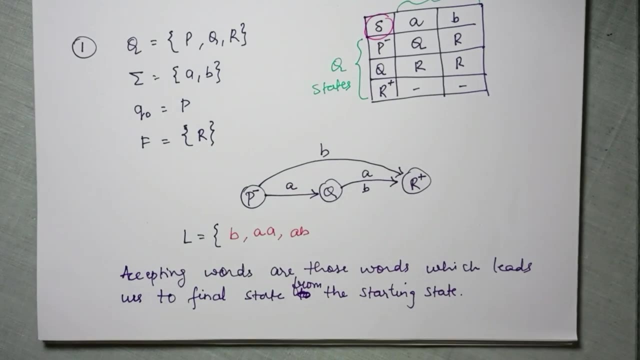 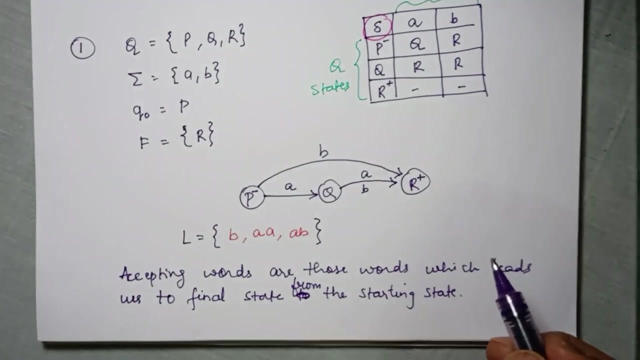 state Hence is accepted in the same way from starting state. if i read a, i go to q. if i read b, i go to r. so a, b is accepted. now, my dear friends, no other word is accepted by this finite automata. so the language accepted by this finite automata is nothing, but it is. 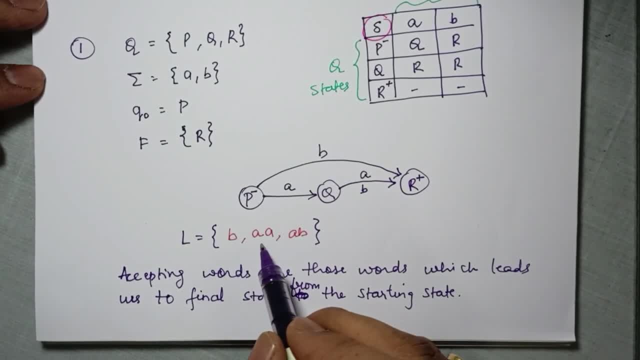 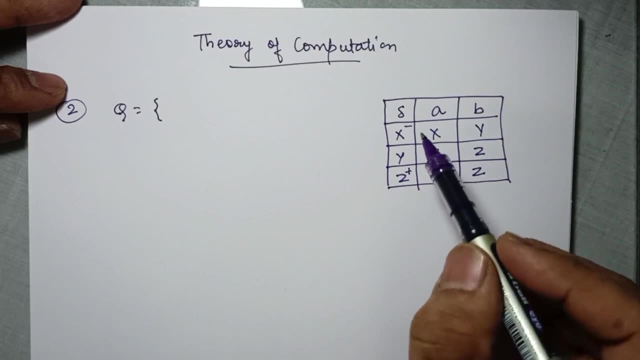 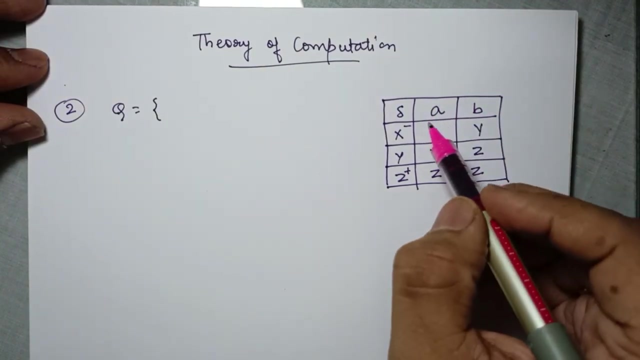 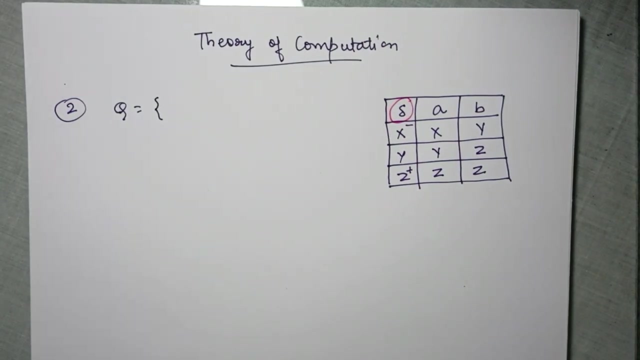 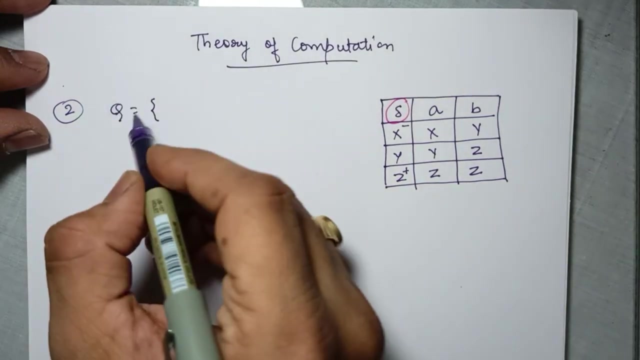 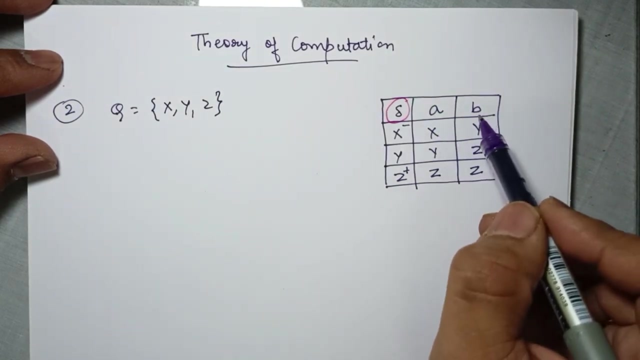 containing three words: b: a, a and a, b. now let us see another example. so, my dear friends, let us see this here: this transition table is given as delta. now we can see this: that this automata contains three states: x, y and z. so my q is then my alphabet set is containing two letters: a and b. 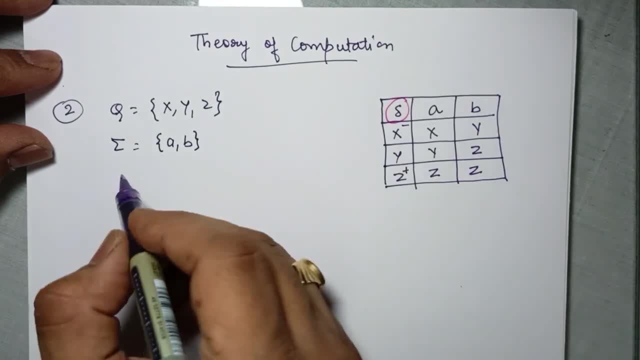 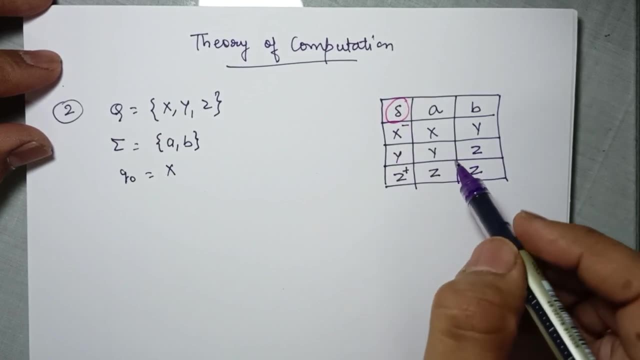 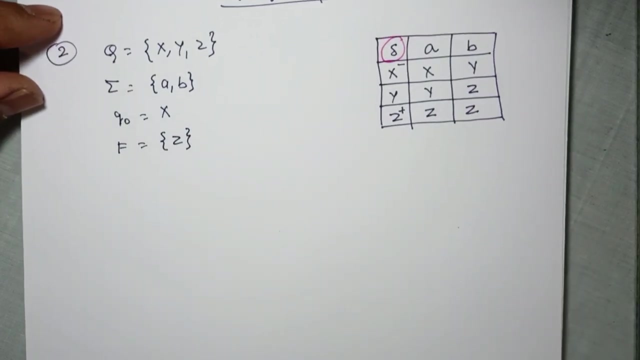 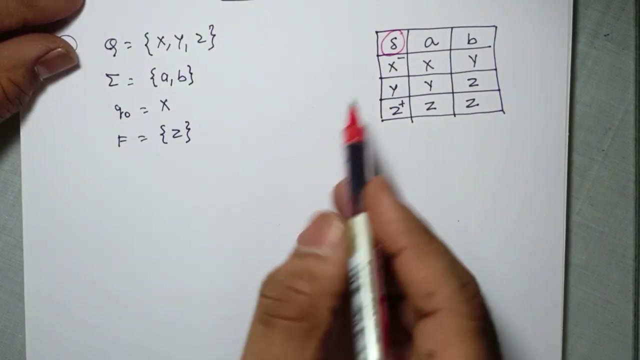 then my starting state here is x, then my transition table is given here with the name delta, then we have the final state. now, my dear friends, let us try and draw the pictorial representation of this finite automata. so there are three states: x, y and z. x is my initial state. 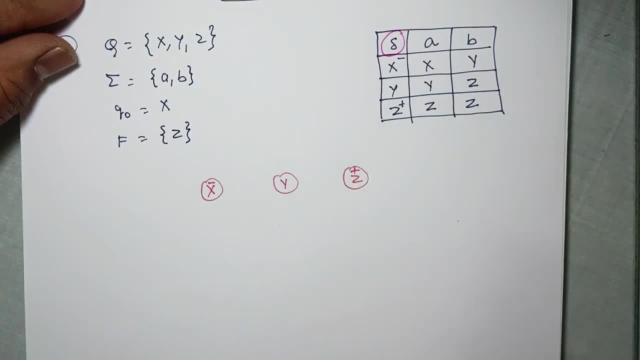 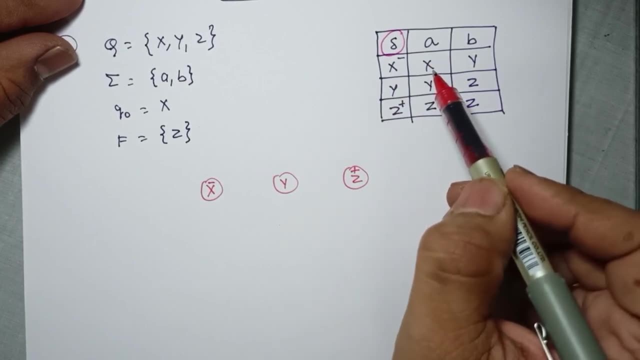 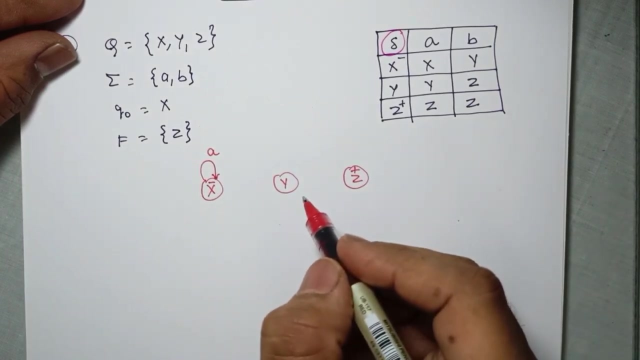 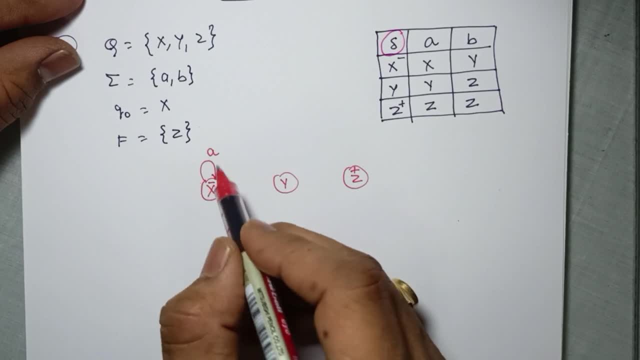 so, my dear friends from x, if i read a, i am going to state x. so, my dear friends from x, if i read a, i am going to state x. so, my dear friends from x, if i read a, i am going to state x. actually, actually, actually this: here you can see that it is remaining in the 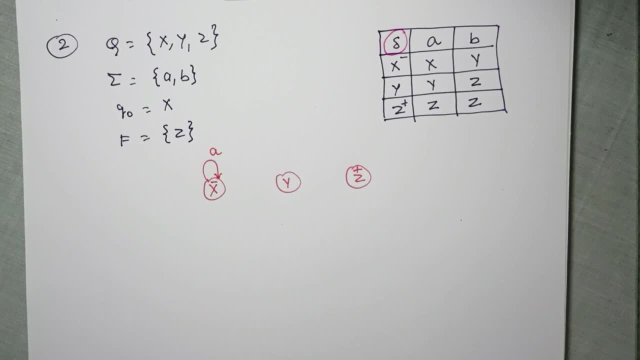 this: here you can see that it is remaining in the. this: here you can see that it is remaining in the same state. so this type of transition, same state. so this type of transition, same state, so this type of transition is called a self loop, is called a self loop. 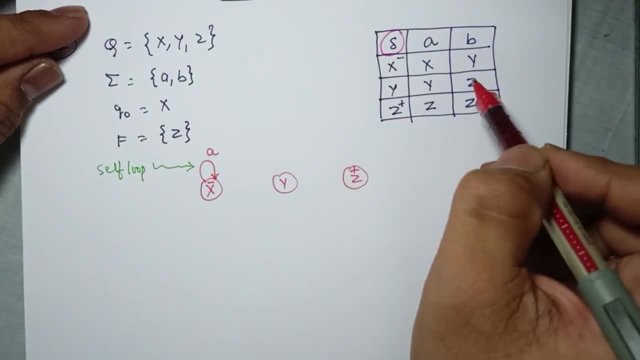 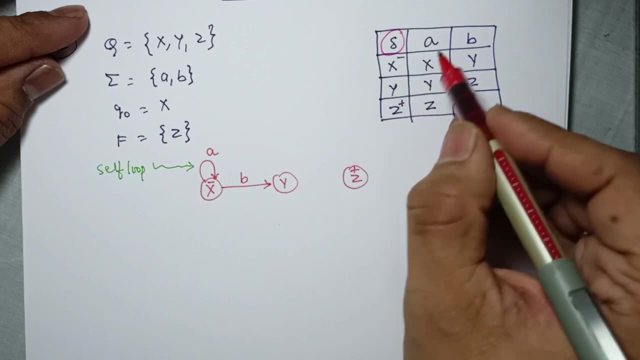 is called a self loop. now from state x. if i read b, i am going to now from state x. if i read b, i am going to now from state x. if i read b, i am going to y now from state y. if i read a, i am going to the. i am staying in the. 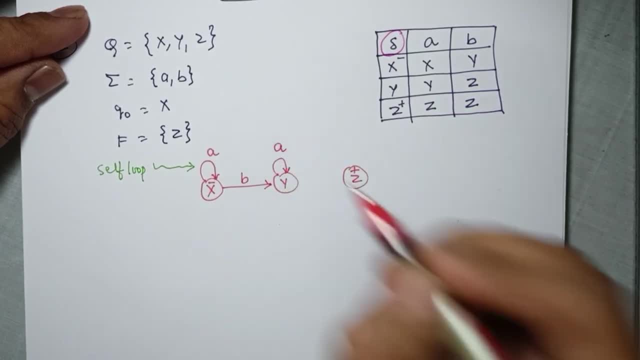 now from state y. if i read a, i am going to the. i am staying in the. now from state y. if i read a, i am going to the. i am staying in the state. state, state y. so again there is a self loop of a y. so again there is a self loop of a. 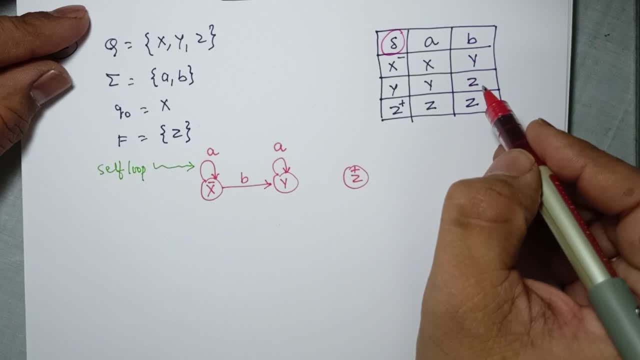 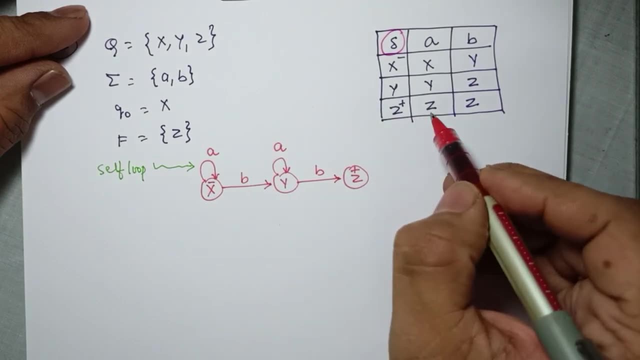 y. so again there is a self loop of a now from state y. if i read b, i am going now from state y. if i read b, i am going now from state y. if i read b, i am going to z now from state z. if i read a, i am staying. 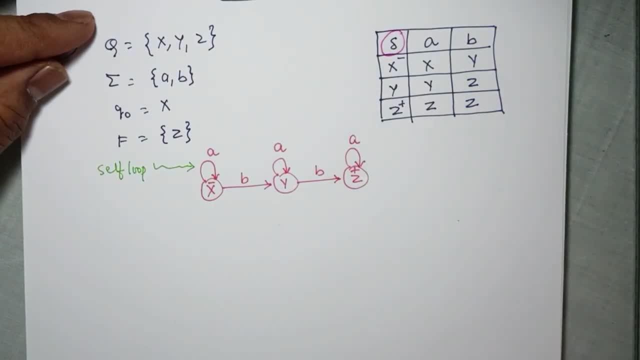 now from state z. if i read a, i am staying now from state z. if i read a, i am staying in the in the in the same state, same state, same state from state z. if i read b, i am staying in from state z. if i read b, i am staying in. 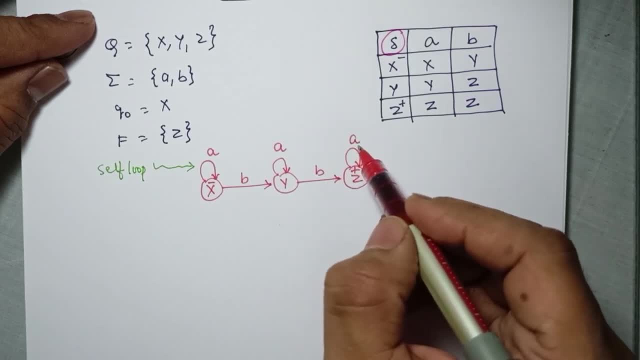 from state z. if i read b, i am staying in the same state. so again i can write this: the same state. so again i can write this: the same state. so again i can write this as a and comma b, or i can draw another as a and comma b, or i can draw another. 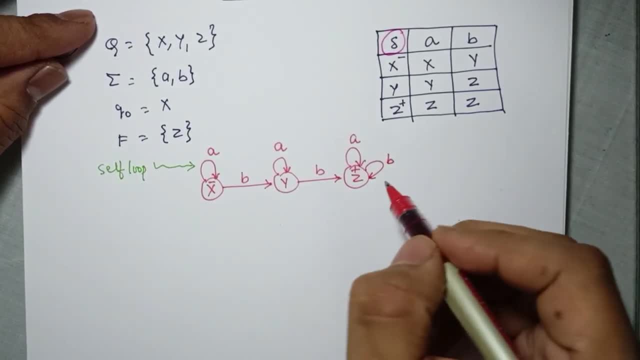 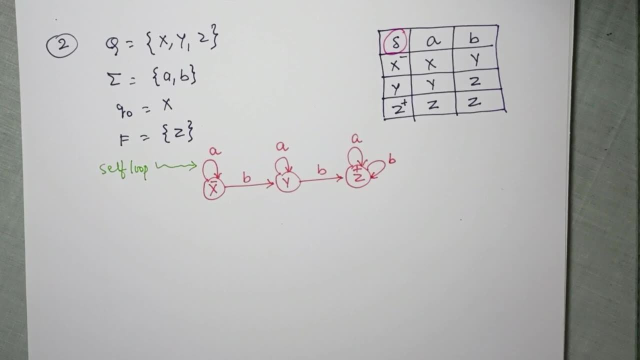 as a and comma b, or i can draw another loop here. it is just a representation. so it is just a representation, so it is just a representation. so this is the, this is the, this is the diagrammatic representation of the diagrammatic representation of the diagrammatic representation of the finite automata. 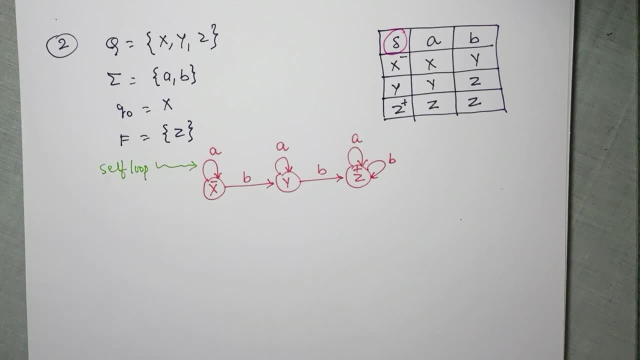 finite automata, finite automata. so again, let us try and have the set of so. again, let us try and have the set of so again, let us try and have the set of accepting words. accepting words, accepting words from this finite automata, from this finite automata. 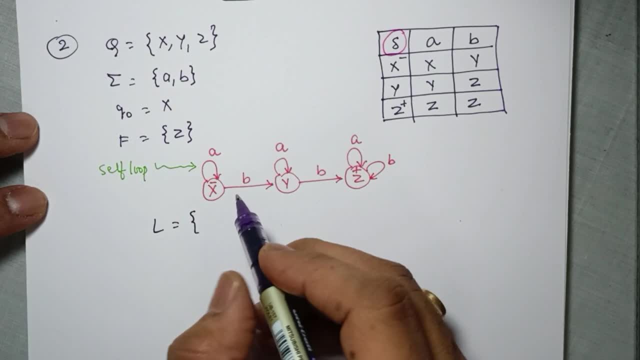 from this finite automata. now, let us now, let us now, let us look at this, my dear friends, look at this, my dear friends. look at this, my dear friends, when you are trying to have, when you are trying to have, when you are trying to have the language that is generated by the 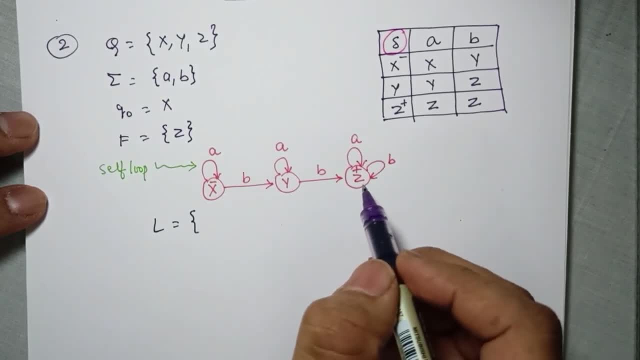 the language that is generated by the, the language that is generated by the finite automata, finite automata, finite automata. you should always start with the minimum. you should always start with the minimum. you should always start with the minimum. word that is accepted. word that is accepted. 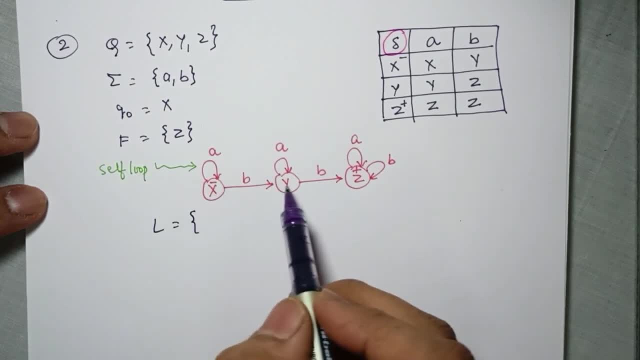 word that is accepted. so here from state x. so here from state x. so here from state x. if i read b, i am going to the state y. if i read b, i am going to the state y. if i read b, i am going to the state y from state y. if i read b, i am going to. 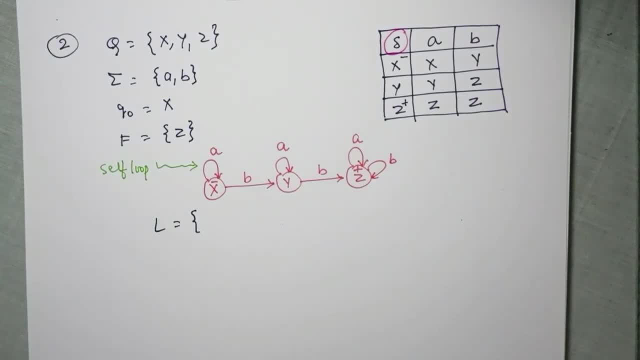 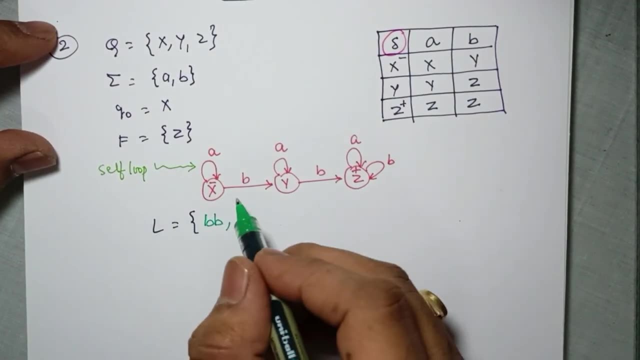 from state y. if i read b, i am going to from state y. if i read b, i am going to the state, the state, the state z. so the word z, so the word z, so the word with letters b b, with letters b b, with letters b b is accepted then. 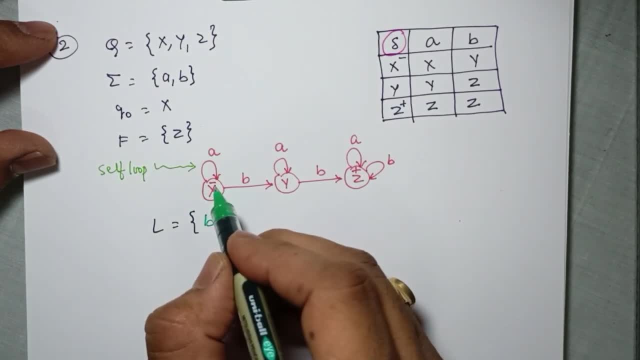 is accepted, then is accepted. then, if i read a, i am staying in x. if i read a, i am staying in x. if i read a, i am staying in x. okay, now understand this very important. okay, now understand this very important. okay, now understand this very important. it is very, very important, my dear. 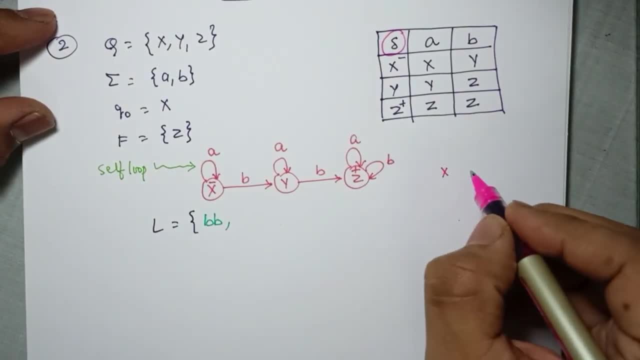 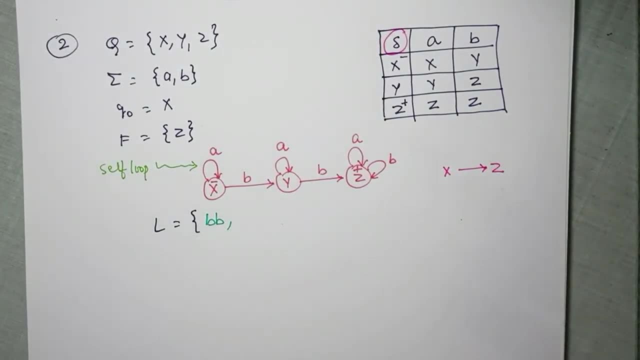 it is very, very important, my dear, it is very, very important, my dear friends, friends, friends. so, from x, so from x, so from x to z to z to z, i have, i have, i have, the bb word accepted. so, if so, if so, if i take it this way, 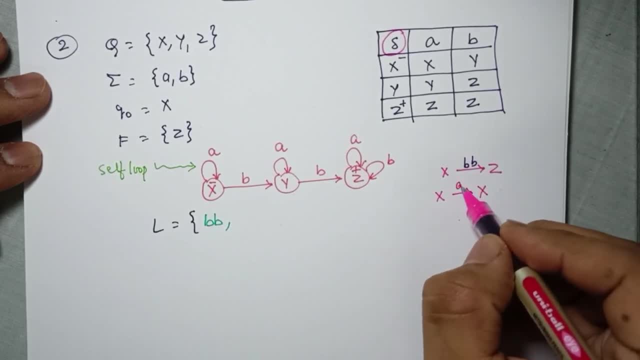 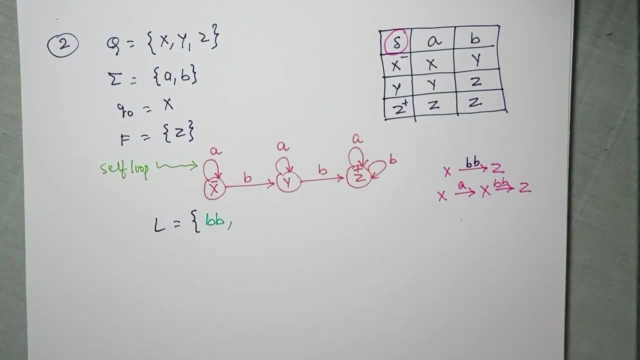 i take it this way. i take it this way: from x, from x, from x to x. i read a to x. i read a to x, i read a, and then from x and then from x, and then from x to z. definitely i have to z, definitely i have. 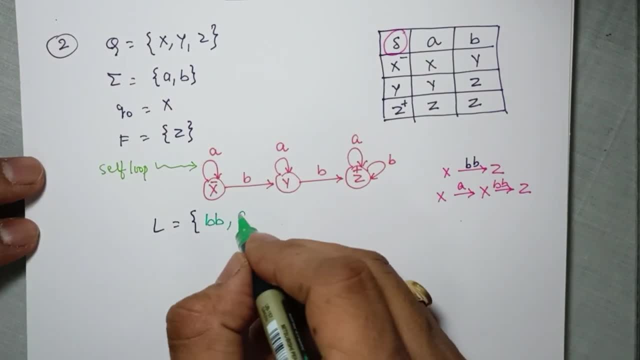 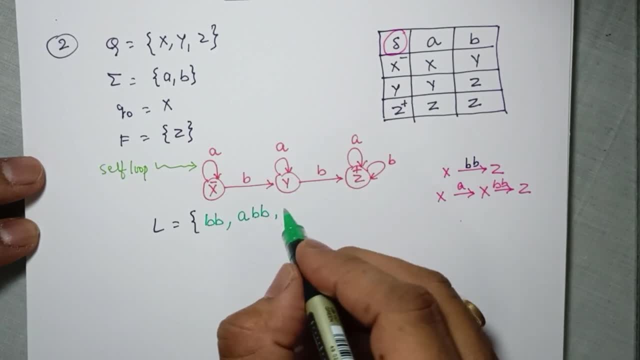 i read here b, i read here b, then i read a, then i read a, then i read a, and then again i read b, so the word, and then again i read b, so the word, and then again i read b, so the word bab is also accepted. 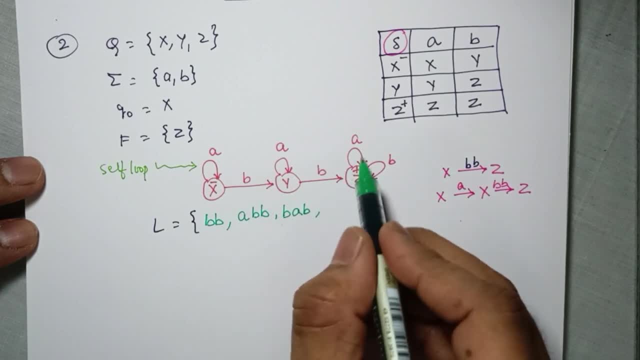 bab is also accepted. bab is also accepted, then then then if i read b, b followed by a, if i read b, b followed by a, if i read b, b followed by a is also accepted, then b is also accepted, then b is also accepted, then b, b followed by b is also accepted. 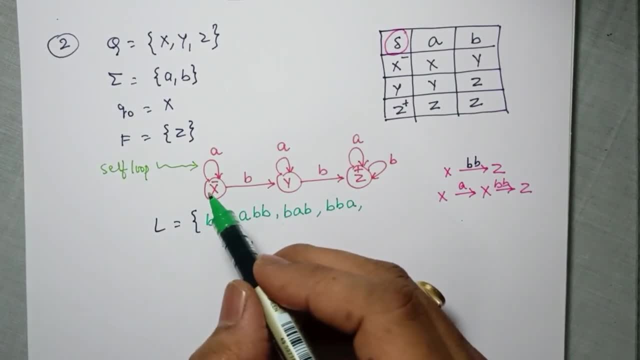 b, followed by b, is also accepted now, followed by b, is also accepted now, followed by b, is also accepted. now this: a since it is a self loop, i can read this: a since it is a self loop, i can read this: a, since it is a self loop, i can read any number of times. any number of times, any number of times. i can read it once. i can read it twice. i, i can read it once. i can read it twice. i, i can read it once. i can read it twice. i can read it. thrice can read it, thrice.